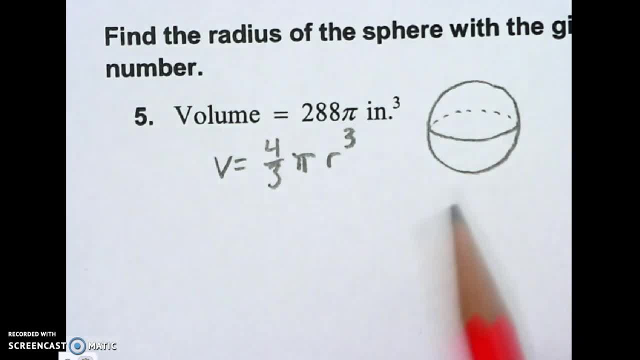 And I did not think it was going to turn out this good. This is a good morning right here, So now I'm going to draw my middle center point and an arrow, a line over to the side. That is r, And that is what we're solving for. 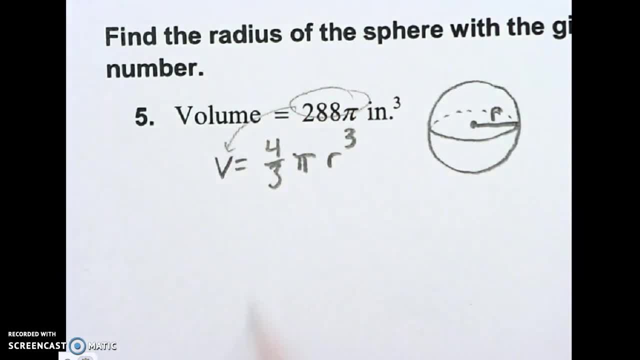 So I'm going to put this volume in the volume spot. So I'll have: 288 pi equals 4 over 3 pi r. If you're wondering what 288 pi means, it's just the 288 and the pi have not been multiplied together yet. 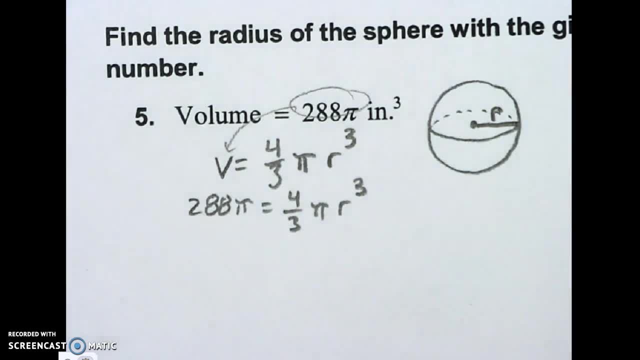 So that's all that's happened there. Okay, I need to solve for r. First thing I need to do is get rid of this 4 thirds and pi. I'm going to deal with the 4 thirds first. If you didn't remember, you can get rid of a fraction by multiplying by the reciprocal. 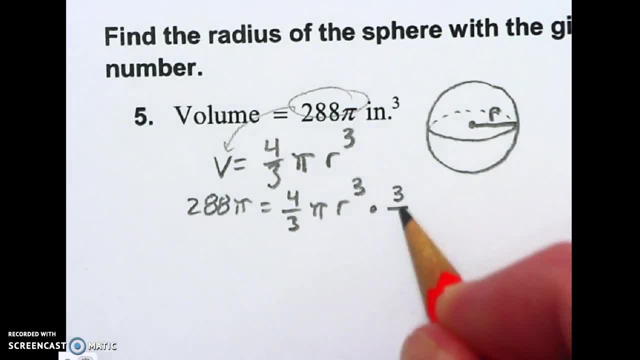 So I'm going to multiply both sides. I'm going to multiply both sides by the flip of that fraction. I'm going to multiply by 3 over 4.. And on this side, I'm going to multiply by 3 over 4.. 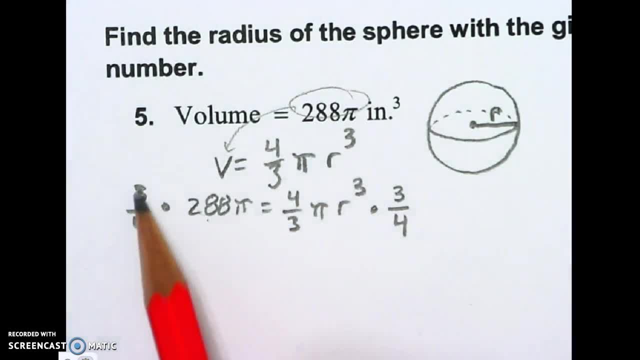 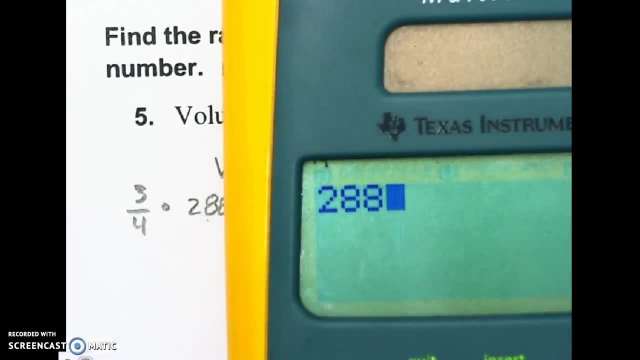 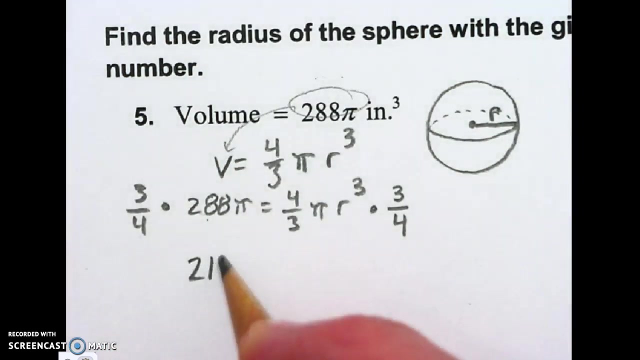 So I'm going to multiply 288 times 3 fourths. Here's how you do that: You do 288 times 3 divided by 4. That's timesing it by 3 fourths, And I get 216.. So this is 216 pi. 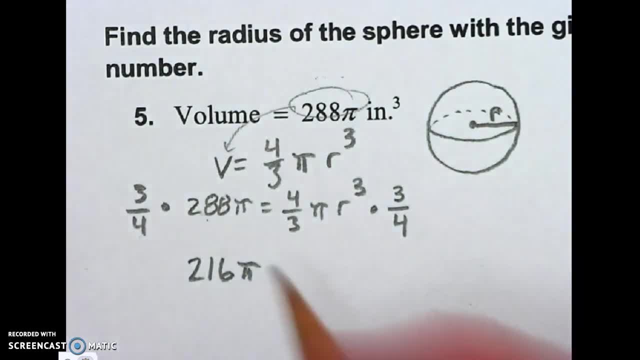 I just left the pi off the calculator because it hadn't been multiplied in, So it's fine to leave it there. And now I have equals pi and r cubed. Notice the 4 thirds went away because we multiplied by 3 over 4.. 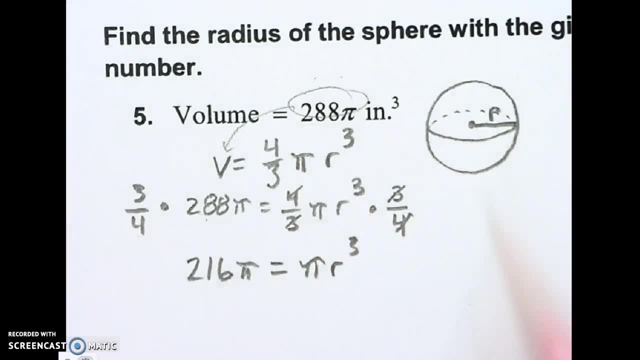 The 3 times been divided, The 4 times been divided, So they canceled out. I got a phone call. It's just going to kind of ring. I'm doing this video, So don't mind it. Next thing I'm going to do is divide both sides by pi. 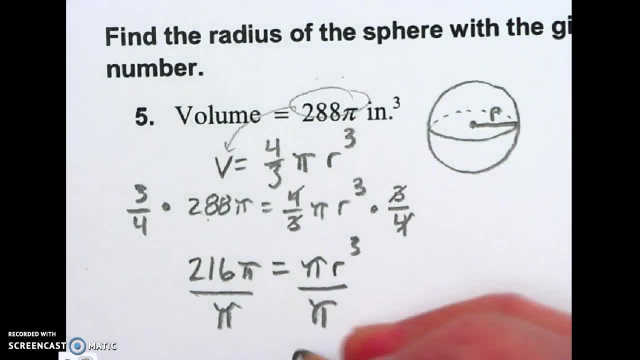 Still ringing. So when I divide by pi, this pi cancels. Kind of cool. There's pi on the other side also, So that cancels. That'll lower my video. There we go, And now I've got just r cubed.